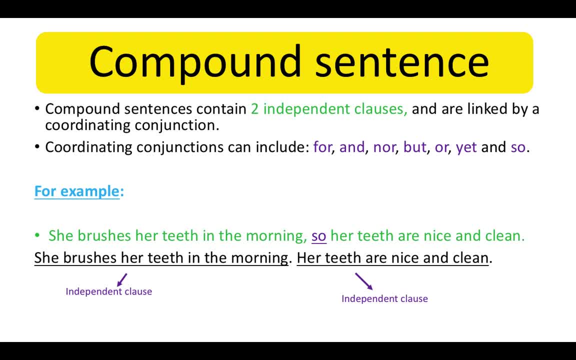 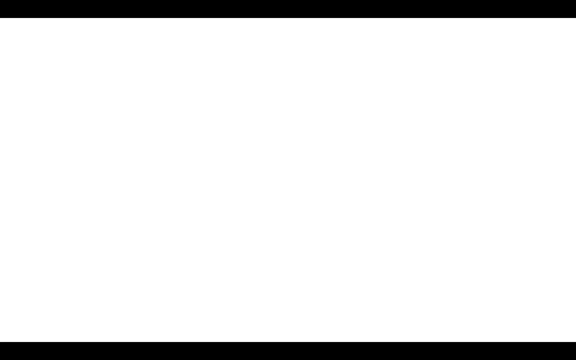 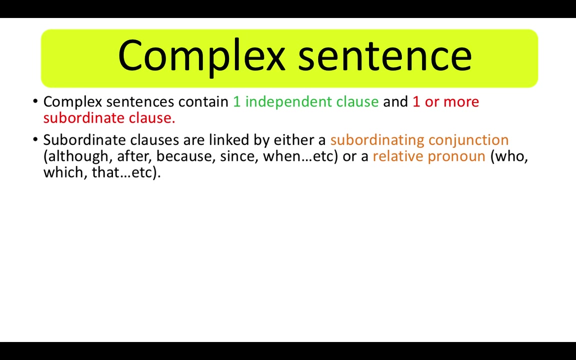 On their own are separate sentences. Another example is: the baby laughed at the cartoon and he played with his toys. It's important to note that we use commas before the coordinating conjunction Complex sentence. Complex sentences contain one independent clause and one or more subordinate clause. Subordinate clauses are linked by: either a subordinating conjunction, For example although, after, because, since, when, etc. Or a relative pronoun, For example who, which, that and many more Examples of complex sentences include: she brushes her teeth in the morning after waking up. 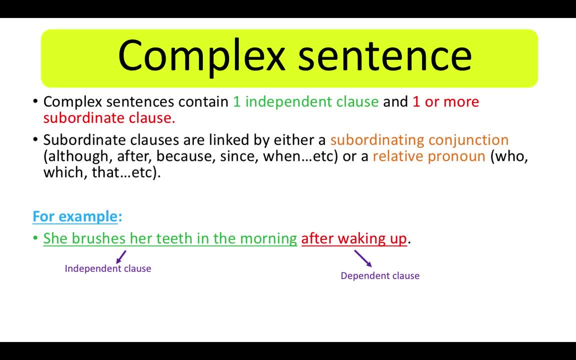 As you can see, we have our independent clause, which can make sense on its own as a separate sentence, and then the dependent clause, which is after waking up. This wouldn't make sense on its own as a separate sentence, so this sentence can't make sense on its own. 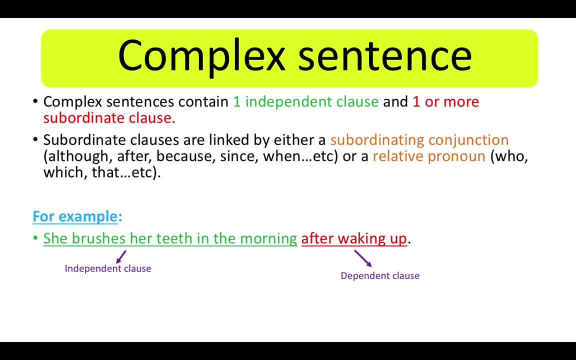 Or we can use my own And I've got the second one. I've got my first one. I've got Devon's. I've got my third one. I've got the third one. I've got Devon's, My third one. 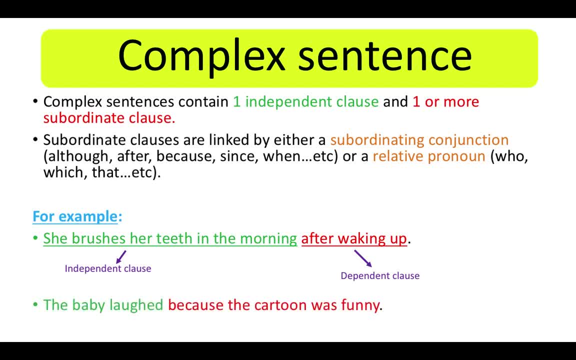 I've got the third one. I've got Devon's. I've got Devon's sentence. The baby laughed because the cartoon was funny. I can't wait to meet everyone at the reunion dinner which is tomorrow. The last example shows you a relative clause with 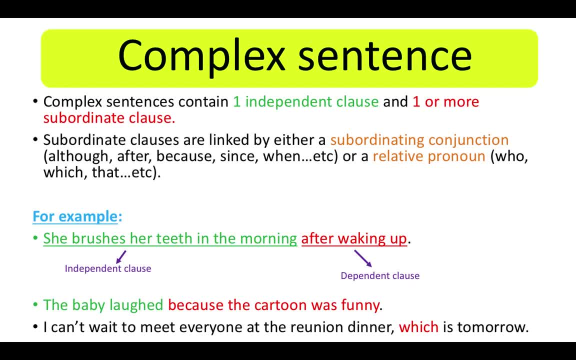 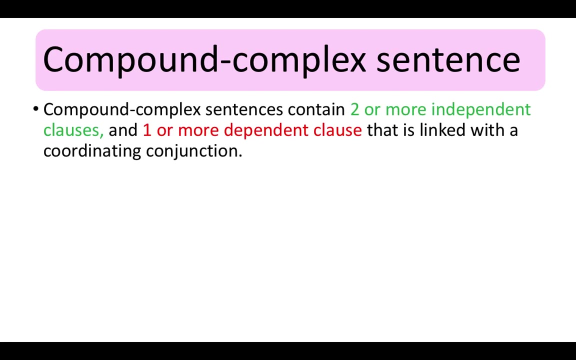 a relative pronoun, which It is important to note, that we use commas when the dependent clause comes first, but if the sentence begins with the independent clause followed by the dependent, then we don't use a comma. Compound complex sentence. Compound complex. 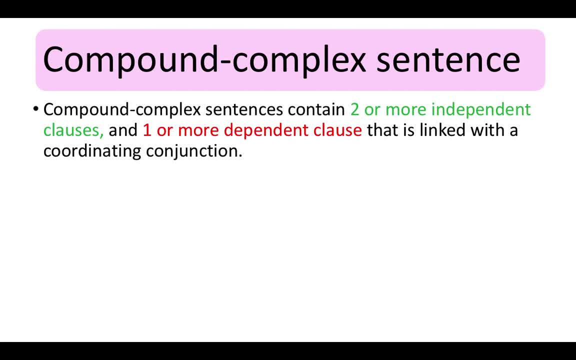 sentences contain two or more independent clauses and one or more dependent clause that is linked with a coordinating conjunction. For example, I woke up in the morning and I brushed my teeth, even though everyone else was sleeping. Here we can see the independent clauses and the dependent clause. 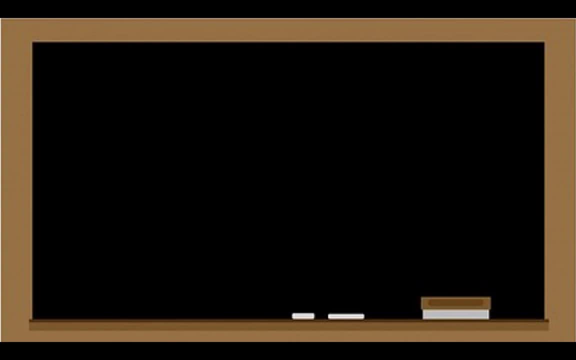 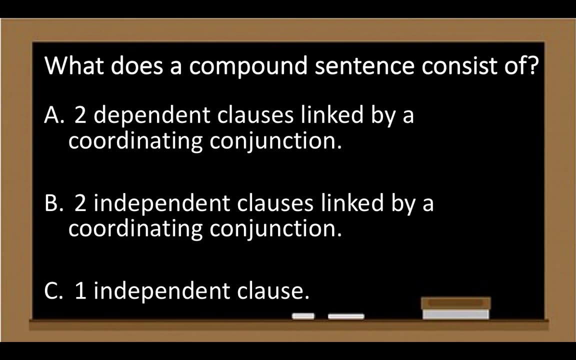 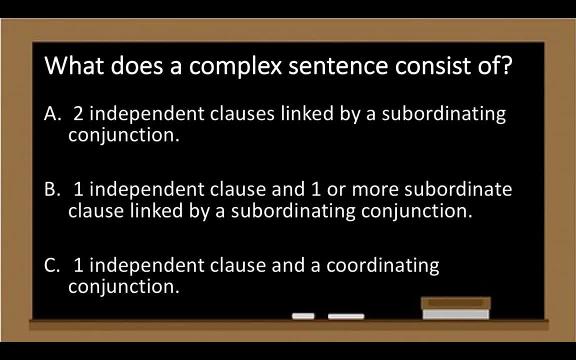 I woke up in the morning and I brushed my teeth, even though everyone else was sleeping.